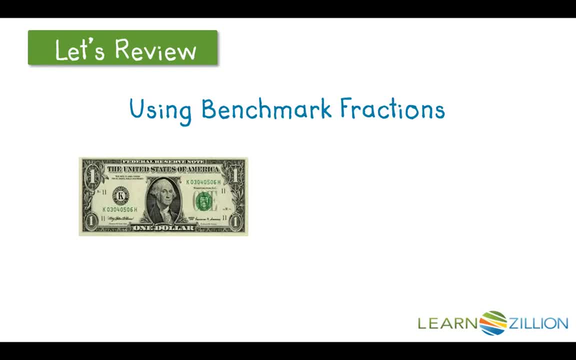 We often think of benchmark fractions in the forms of money, But we can also think of fractions in terms of almost Three fourths is almost one whole. Twelve, fourteenths is almost one whole. Thirteen, forty-eighths is almost one fourth. 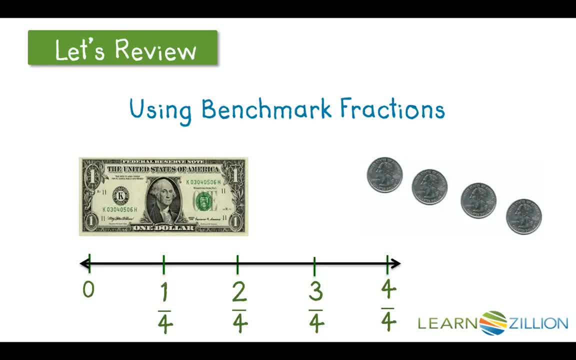 The dollar idea gives us a great everyday way to think about benchmark fractions such as one fourth, one half and three fourths. We will use this idea in this lesson to work with benchmark fractions as a way to estimate for the reasonableness of our answers in story problem fractions. 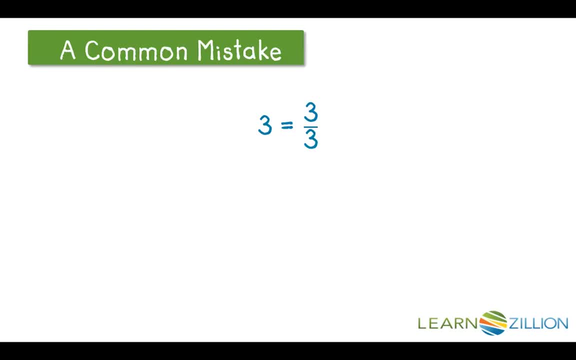 A common mistake that some students make is representing the whole number three as three over three. As you can see, the whole number three would be modeled as three whole parts in a number line. You can also see that three out of three means that there are three parts of one whole. 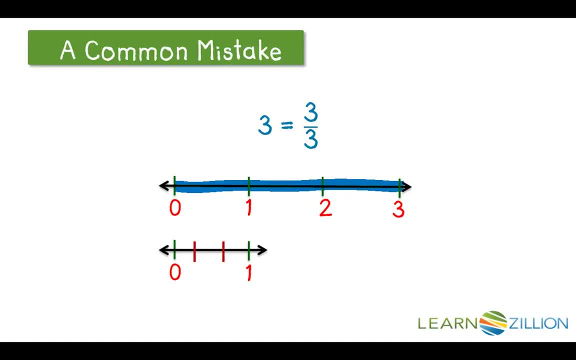 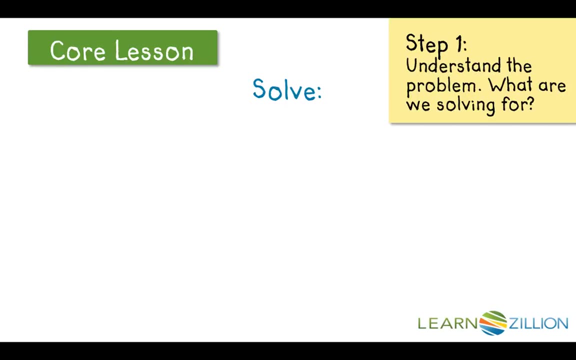 with all three parts shaded in, which totals one whole Let's solve, Discuss with students that there are four main steps in solving any story problems. In step one, we read the problem carefully, maybe even twice. We underline, highlight or circle. 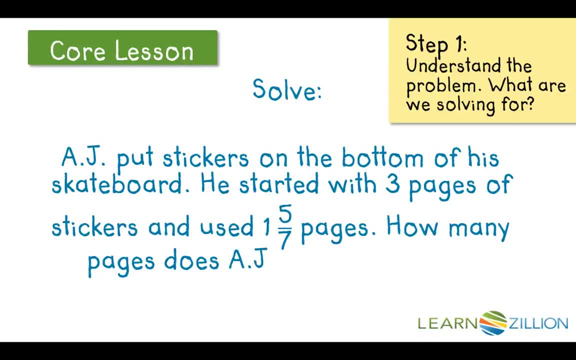 important information. We can also eliminate any unnecessary information In step one. we want to make sure that we understand what the problem is asking and what are we solving for. In this case, the problem is asking us: how many pages does AJ have remaining? 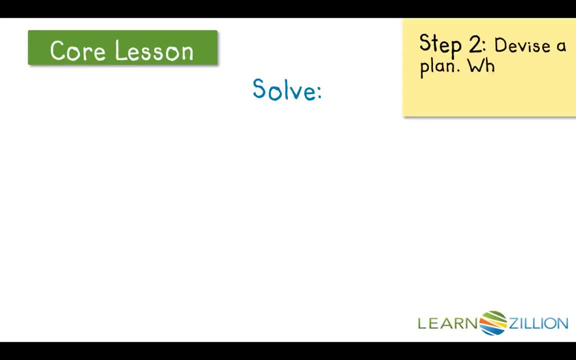 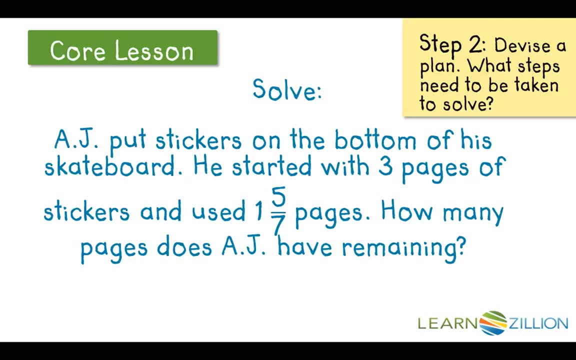 Now that we understand what we're solving for what steps do we need to take to solve? What data is given? What keyword in the story problem tells us which calculation we will use? Great job. We now know that we need to subtract one and five sevenths from three. 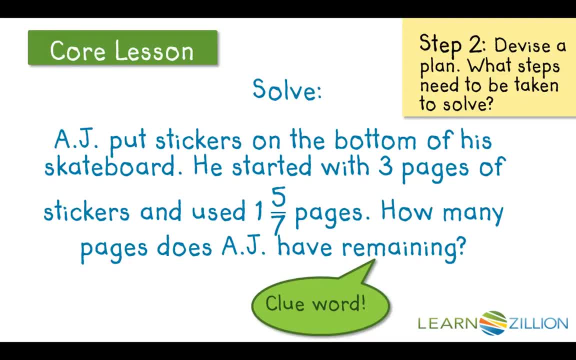 to answer this question, We can estimate one and five sevenths to be one whole and nearly one more whole, since five out of seven shaded would be more than one- half our benchmark fraction. We can also think that three and a half out of seven would be half.